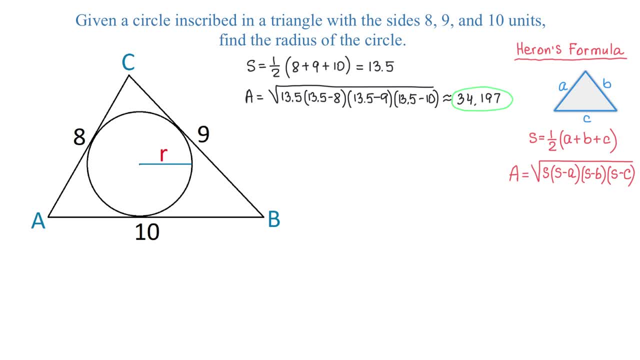 in this figure. first we will need to connect a few points In this figure. first we will need to connect a few points. Let the center of this circle be represented by letter O. Now we will connect point O with the points A, B and C. 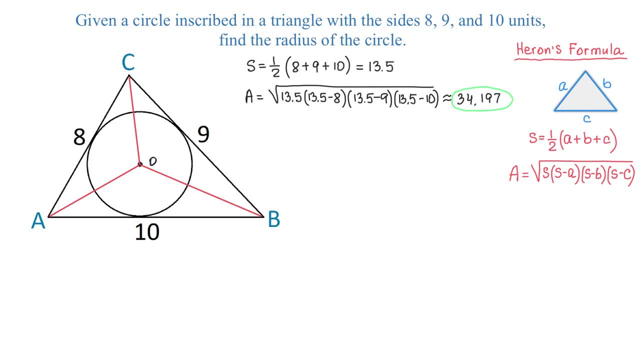 Now, the sides of the triangle are tangent to this circle and these are the points of tangency. If we connect the center of the circle with each point of tangency, then each of these line segments will be perpendicular to each side of the triangle. 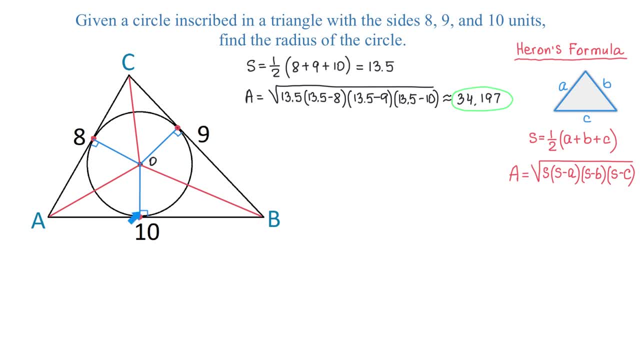 So here I have them connected, and each of these line segments also represents the radius of the circle. And now let's take a look at the triangles AOB, BOC and AOC. These triangles together form the triangle ABC. In the triangle AOB, the base is 10 and the height is R. 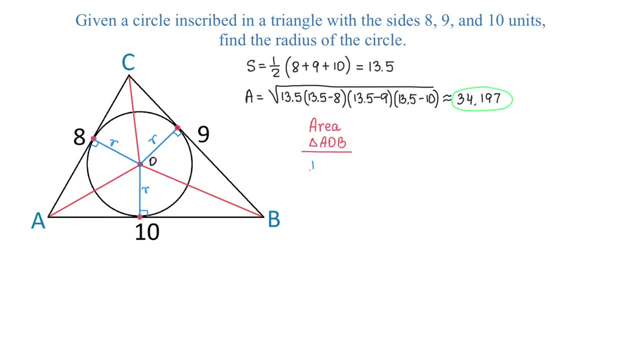 Then we can say that the area of AOB is 10.. Then the area of this triangle is 1 half times the base 10 and times the height R, And if we simplify this expression, that will be 5R. Now in the triangle BOC the base is 9 and the height is R. 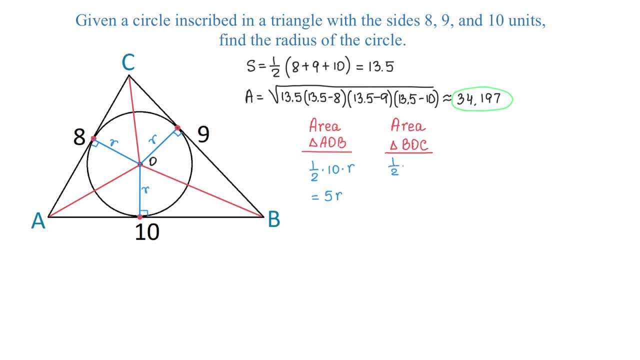 Then the area of this triangle will be 1 half multiplied by 9 and multiplied by the height R, Then this equals 4.5R. And now Now in the triangle AOC, the base is 8 and the height is R. 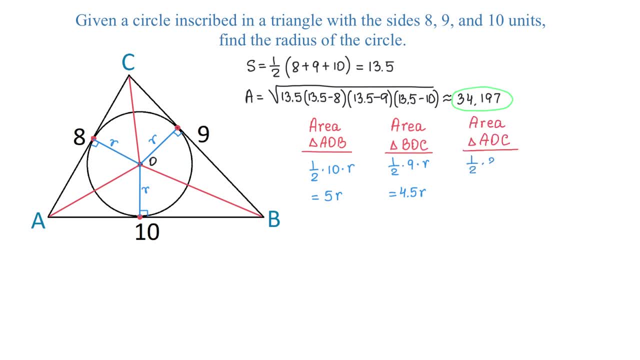 Then the area is 1 half times the base 8 and times the height R, which equals 4R. And now if we add these areas together, we will get the area of the triangle ABC. So 5R plus 4.5R plus 4R. 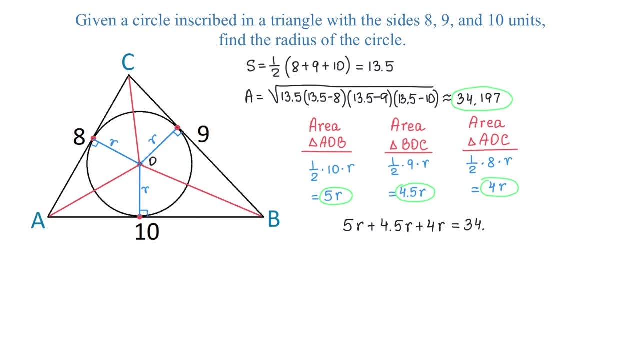 Equals 34.197.. Now if we solve this equation, then we will get the radius of the circle. On the left side we will have 13.5R and on the right side, 34.197.. Let's divide both sides by 13.5..